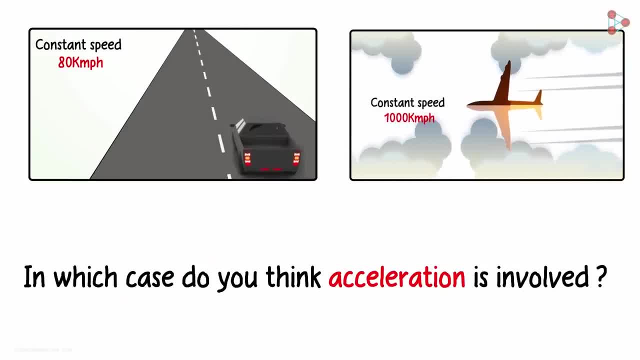 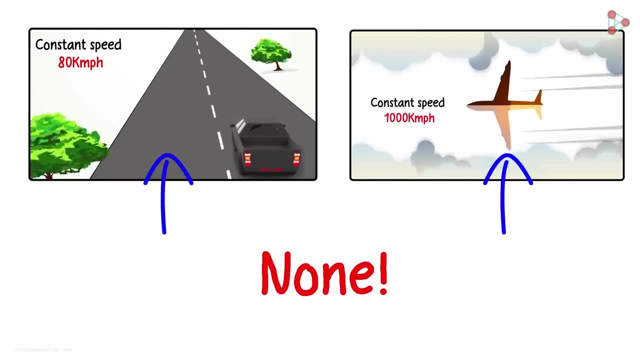 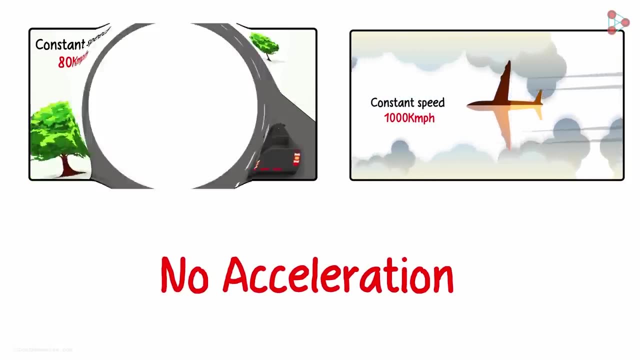 In which case do you think acceleration is involved? None, In both cases, the velocity is not changing at all. Hence there will be no acceleration in either of the cases. Most people relate acceleration to high speed, And that's clearly not true. 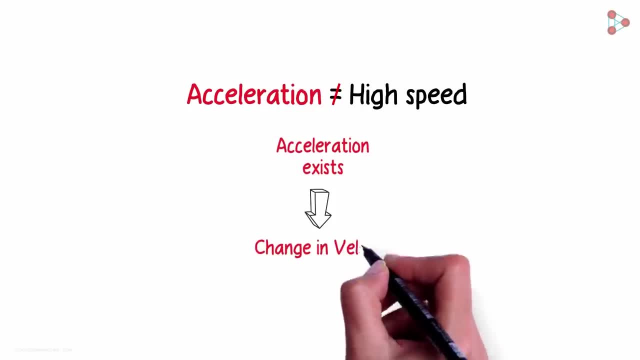 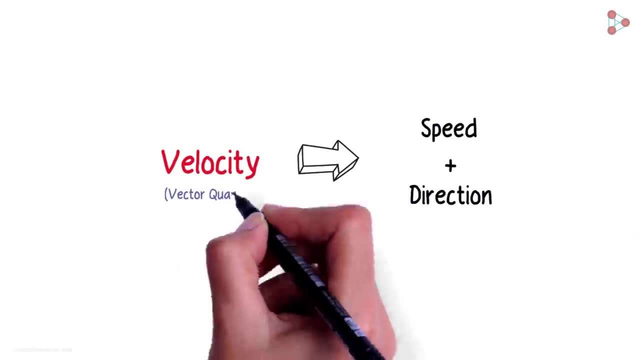 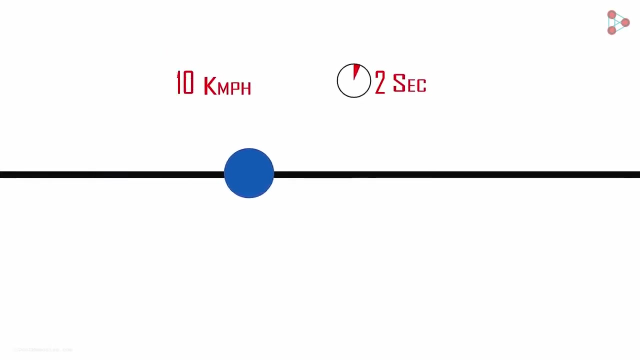 Acceleration will only exist when there is change in velocity. Do you remember what velocity is? It's speed with direction, and it's hence a vector quantity. Why is this important? Let's say, a body moves from rest and reaches a velocity of 20 km an hour in 5 seconds. 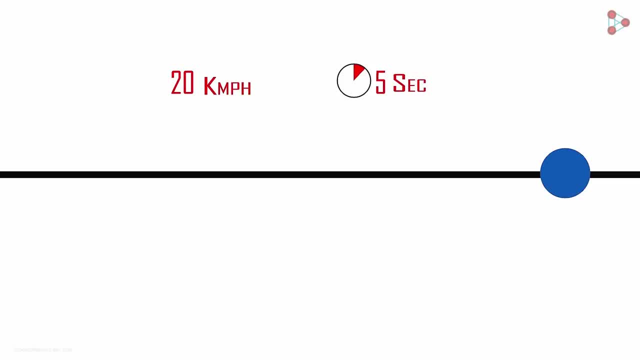 Will acceleration be involved here? Yes, because the velocity is changing. It was zero initially and at the end of 5 seconds it's 20 km per hour. In another scenario, assume that a body is moving at 30 km an hour. 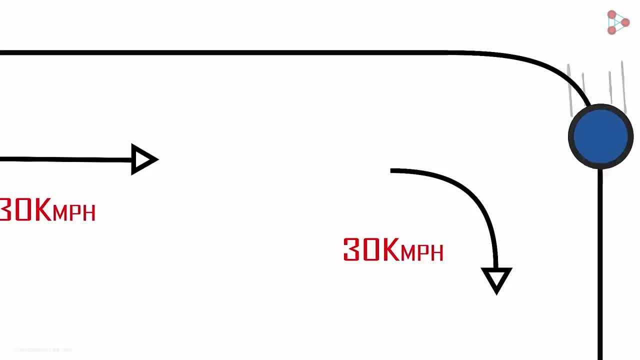 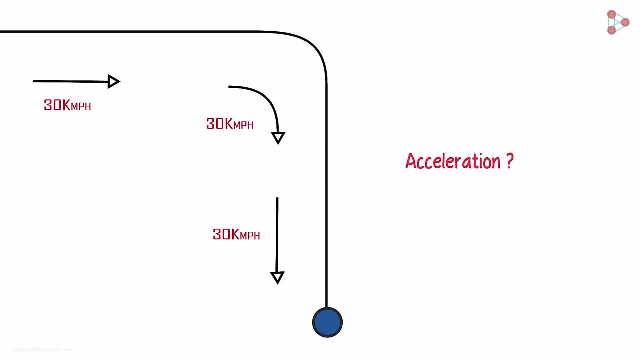 And then it moves right at 30 km an hour and continues traveling at the same speed of 30 km per hour. Will there be acceleration in this case? The answer is yes. As the direction is changing, the velocity will also change. The only thing constant in this example is speed. 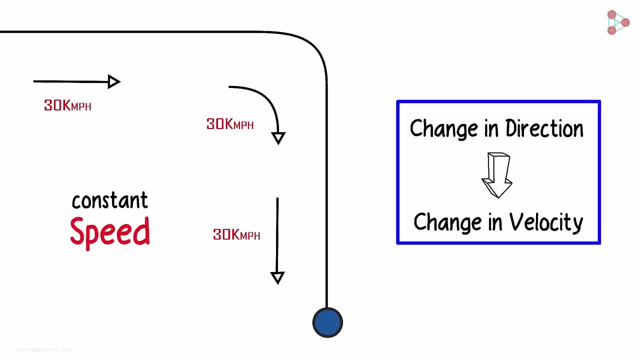 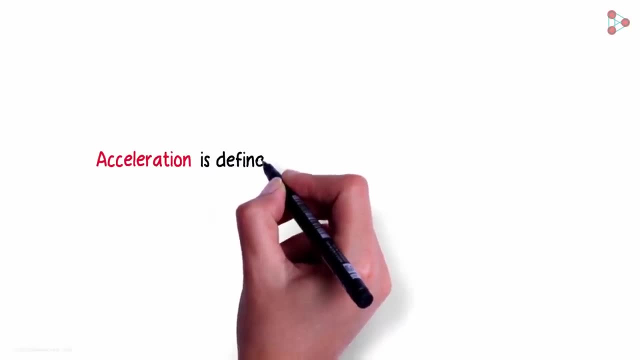 But the velocity changes as the direction changes. So this was the most important concept you had to know about acceleration. It will exist only when there is a change in velocity. But how is acceleration calculated? Acceleration is defined as the rate of change of velocity. 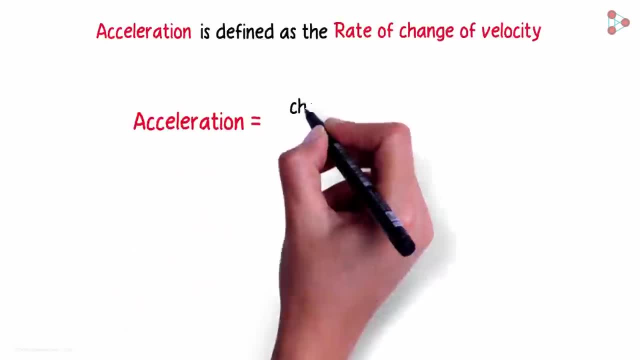 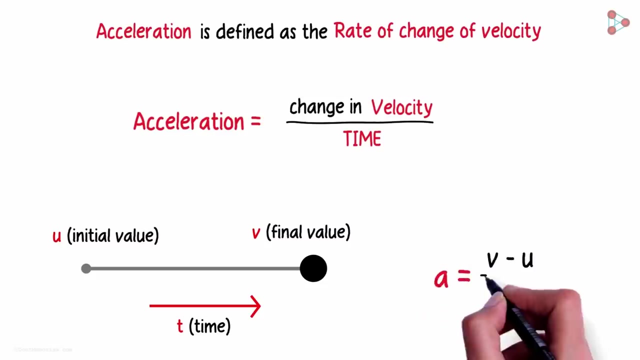 In terms of a formula. acceleration can be written as change in velocity over the time taken. If the velocity of an object changes from an initial value of u to the final value of v in time t, then the acceleration a can be written as v minus u over t. 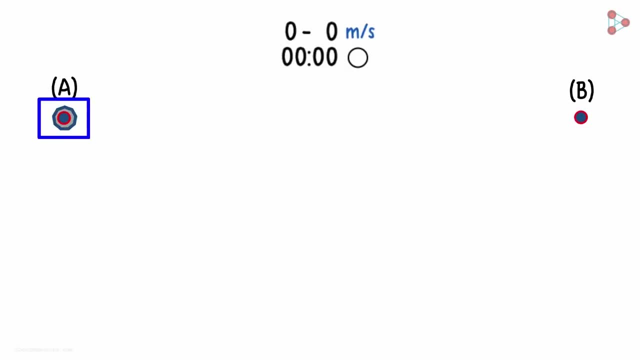 Say: this object is at rest initially at point a. It then travels to the right and attains a velocity of 10 meters per second in 5 seconds. What will be the acceleration here at point b? We can look at the formula to get the answer.